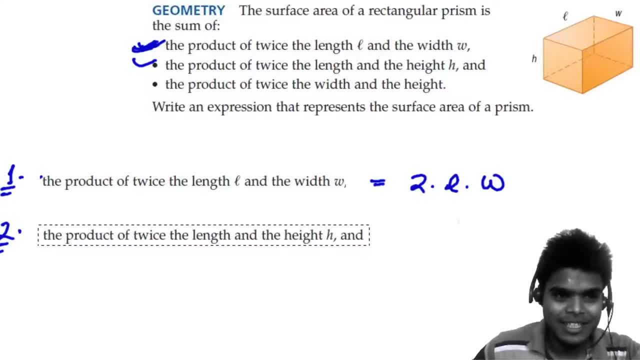 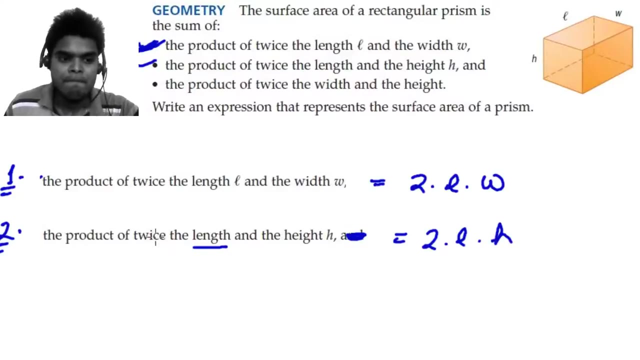 Smart boy. All right, So the product of the twice the length and the height. All right, We don't need this. So, two times the length: Okay, the length which is L and the height which is H. Okay, now the third one, which is the product of the twice the width and the height. All right, then I have to copy this, to copy and then paste. 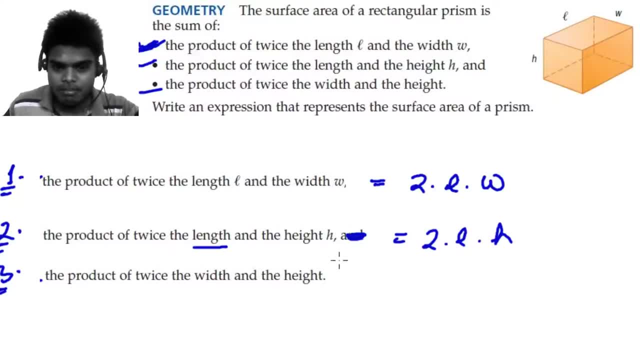 All right, So the product of the twice the width and the height. two times it means. two times product means multiply right Width and the height, Okay, And as the question is saying, the surface area of the rectangular prism is the sum of this, Okay, so therefore, we're going to add everything. This is all we're going to add, All right, Okay, so the expression for surface area of the prism. 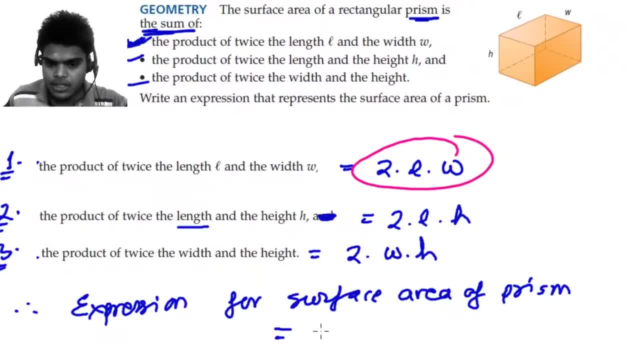 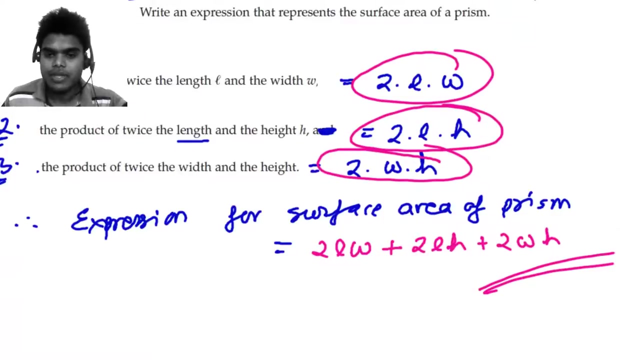 Is equals to, we have to add everything. Okay, First let's do that to LW- This dot you can remove, Okay, And then plus this one to LH, And then this one to WH to WH. Okay, here L represents the length, W represents the width and H represents the height. So this is the algebraic expression for the surface area of the prism. I hope you understand All right. In the next video I will show you some 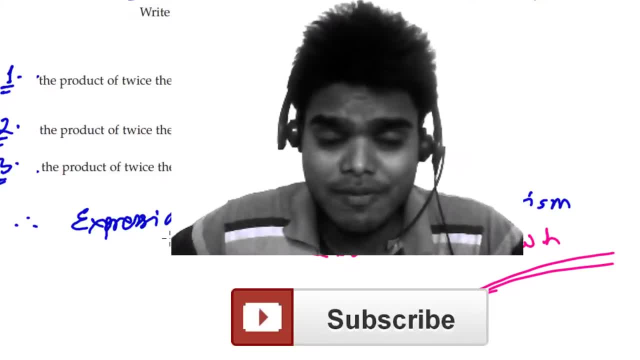 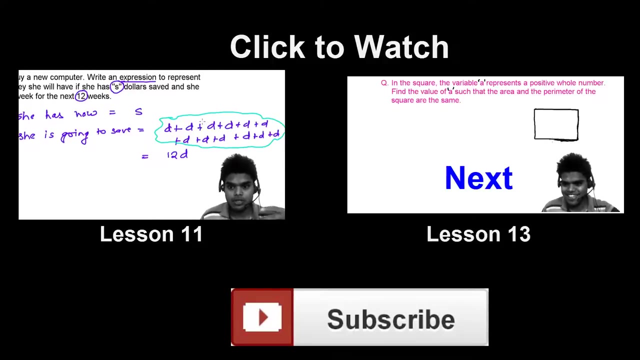 more cool examples, And please don't forget to subscribe the channel. Catch me on Facebook. And hey, if you like my videos, please support me. Subscribe this channel. Catch me on Facebook. Twitter. I will update there too. Okay, Every, every video updates. This is the world's best square, Okay. So the the side length of the square is a. you know already that the every side of the square is of same measurement, Okay. 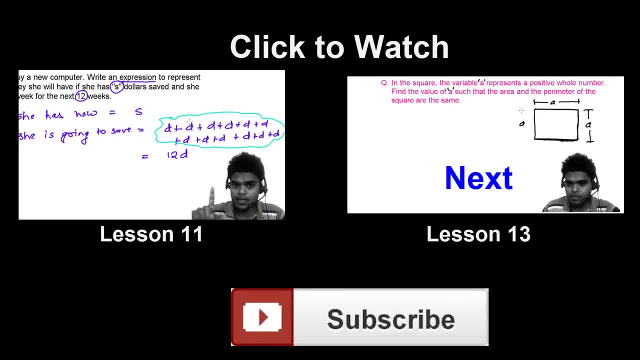 Which, according to the question here, is a. All right, So now the question is saying us that in the square, the variable A represents the positive whole number. Okay, Positive whole number means: